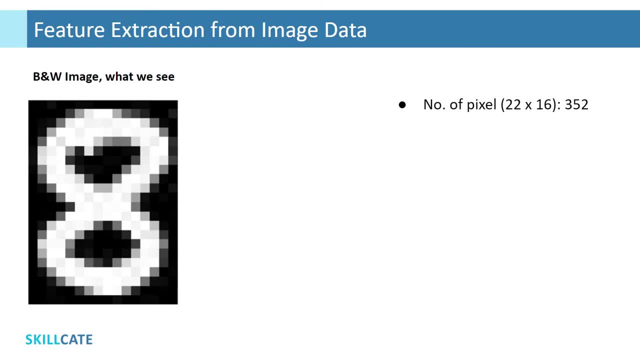 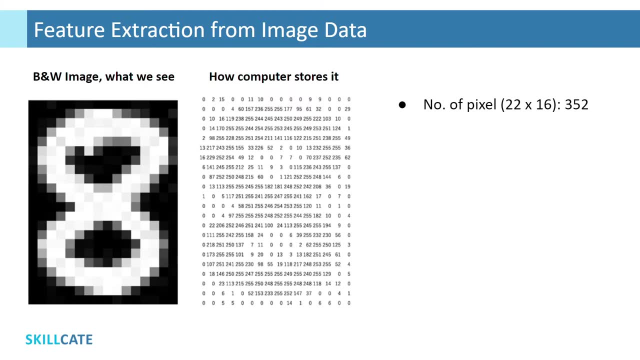 may observe that it's a number 8.. But the question is: how would a computer know that it's a number 8?? The answer lies in how a computer stores this image, data, which is basically a matrix. This particular image has a size of 22 by 16, meaning there are 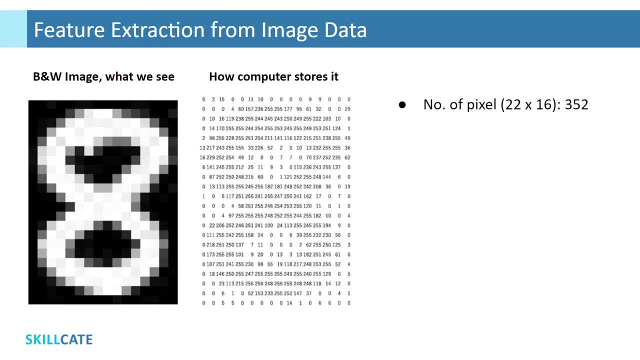 22 pixels along the height and 16 pixels along the width, And in totality there are 352 pixels. A computer stores a number between 0 and 255 for each of these 352 pixels, And this number is a measure of the respect to the image. 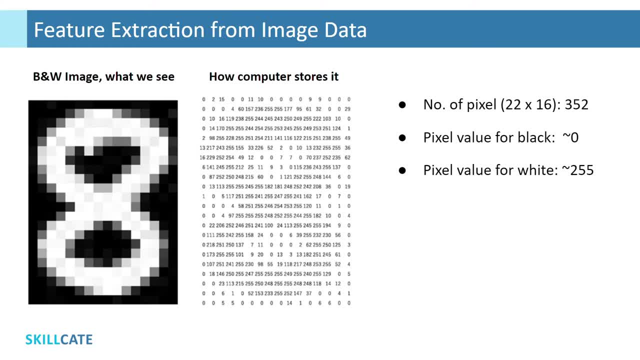 Let's take a look at the image by using the definition of a number. Let's take a look at the definition of a number in the image. For example, if we want to measure the height of an image, we can do so by filling in an. 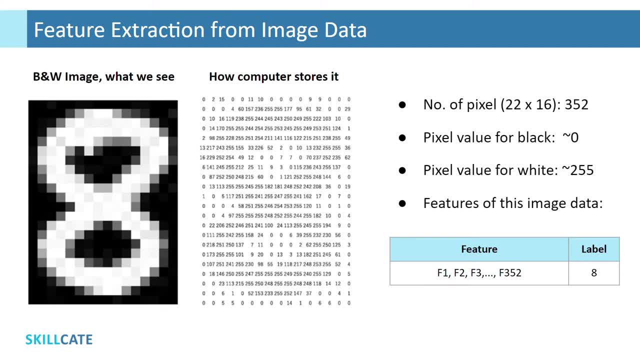 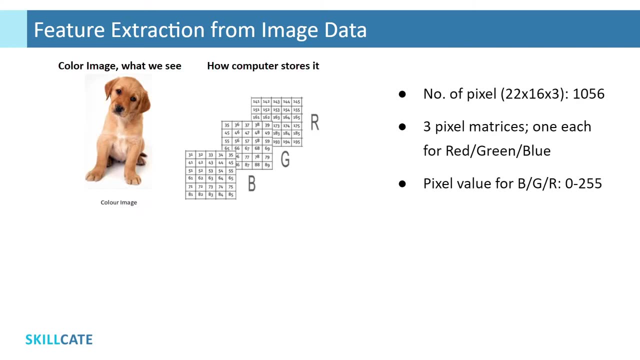 image with a number, So we can always measure the height and width of this image by adding an extra value to it. So this number is the number of pixels that is being calculated to measure the height of the image. For the image key we have a number and a number that are related to the value And. 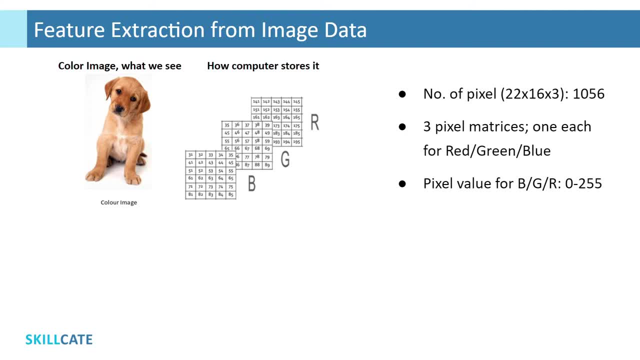 The computer would store three pixel matrices, one each for blue, green and red color intensities, Again on a scale of 0 to 255, depending on brightness intensities. We may replicate the previously discussed approach for black and white image here as well. 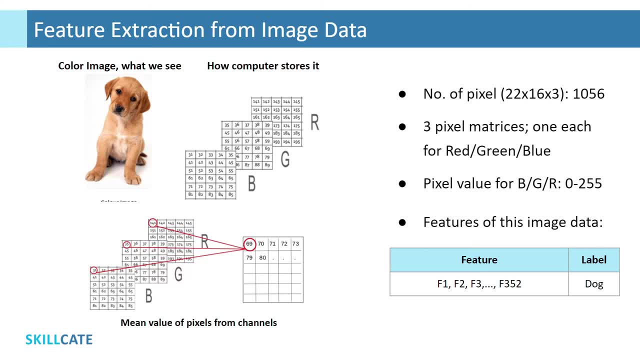 For that we simply need to prepare a new pixel matrix carrying mean pixel values for corresponding pixels from the three matrices which are called as channels. Further steps are the exact same as discussed previously. While this approach of feature extraction from images is simple, it is prone to a lot of problems. 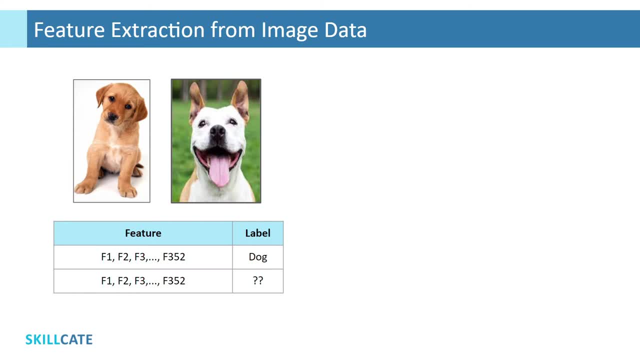 Consider. we are comparing these two images. We have extracted features for these using our simple approach. As we may observe, this second image has a background, while the first does not. Also, the color of the two dogs are varied. And not just that, even the expressions of the two dogs are different. 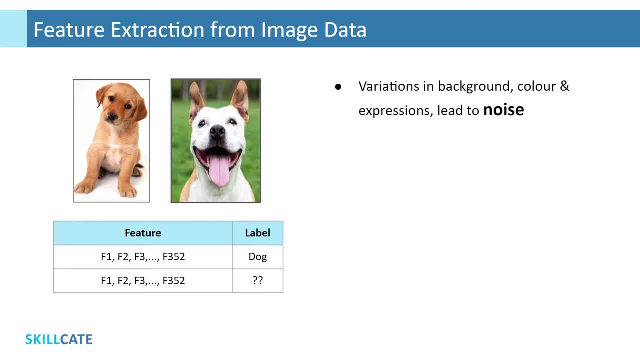 All these factors are collectively called as noise. A good feature extraction approach would tend to minimize this noise, And clearly our simple approach cannot do it, as it directly uses image pixel intensities. Not just that, our simple approach is computationally expensive, as it retains so much unnecessary information. 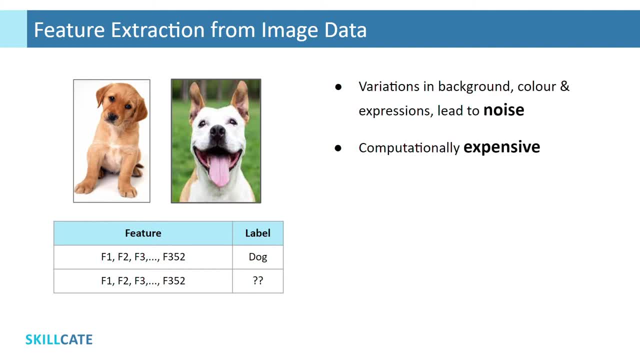 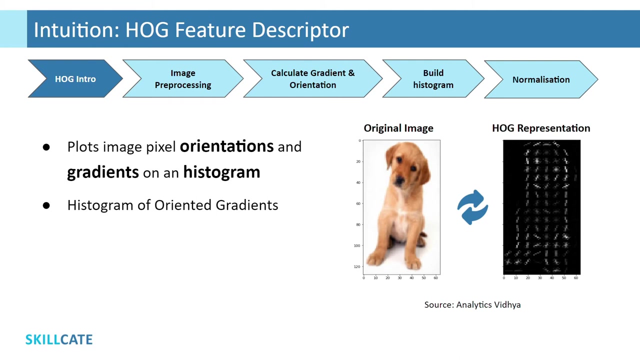 that a good feature extraction approach may otherwise drop. Hence we need a more systematic approach to extract features from images, an approach that retains only the crucial information while discarding the rest. For achieving this, we use HOG, feature descriptor. Simply put, HOG computes pixel-wise gradients and orientations and plots them on a histogram. 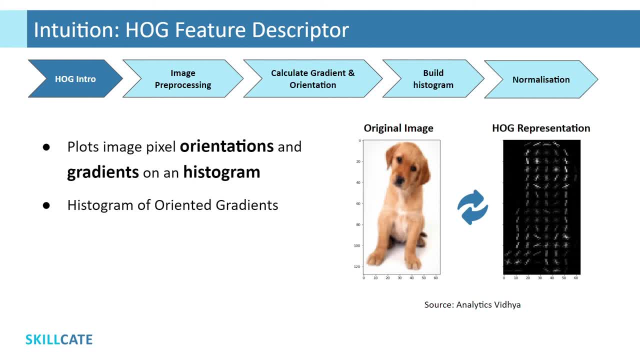 And hence the name Histogram of Oriented Gradients For this original image. this is the HOG representation. As we may observe, HOG has simplified representation of this image, drastically retaining only the most important information. This way, HOG is able to minimize overall noise here. 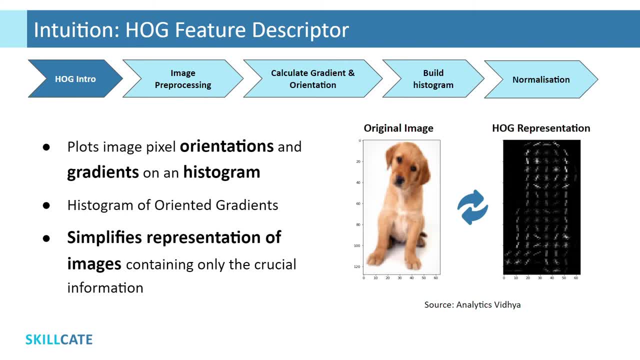 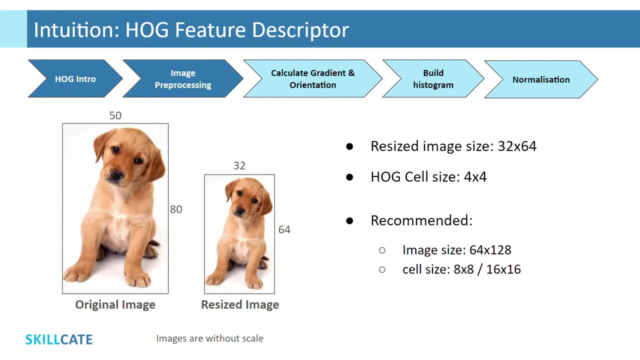 In the coming slides we would go step by step into building this HOG representation for this sample image. We would try to cover the in-depth intuition without going too much into technicalities. First step is image pre-processing, wherein we would standardize image size. 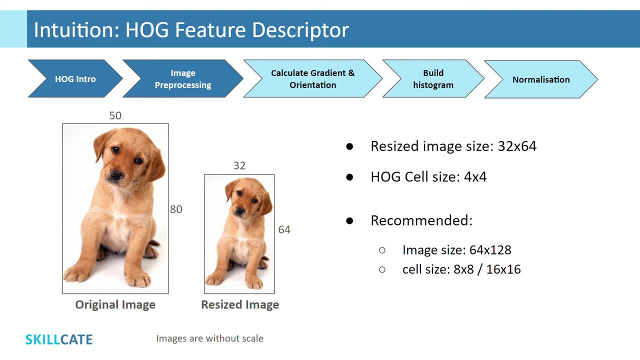 When we are building a face recognition machine learning model, we are feeding tons of images for training our model And it is very important for us to ensure all images are of equal size. In our case, we are running a very long process of training our model. 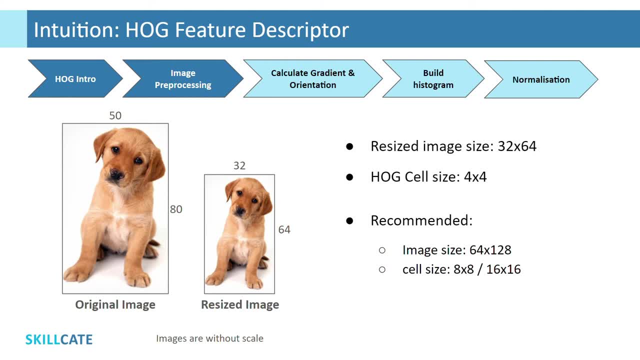 And it is very important for us to ensure all images are of equal size. In our case, we are running a very long process of training our model And it is very important for us to ensure all images are of equal size. We are resizing our images to 32x64.. 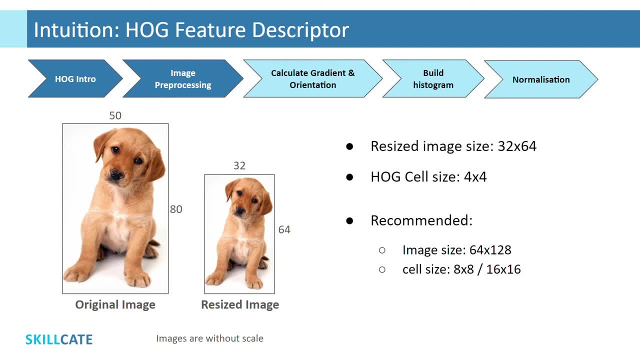 This means we are having 32 pixels along image width and 64 pixels along image height. Next up, we would divide our resized images into 4x4 cells for calculating gradients and orientations, which we would discuss next. Just to highlight here, it is recommended to resize the images to 64x128,. 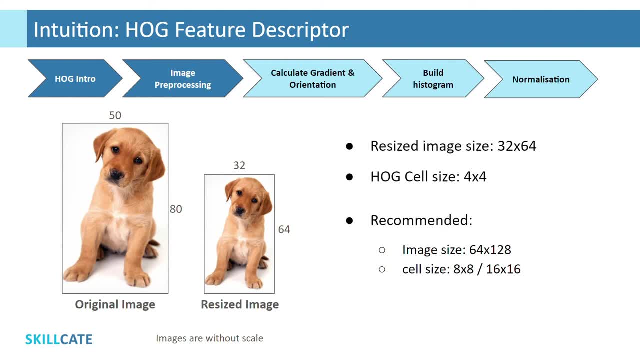 Just to highlight here: it is recommended to resize the images to 64x128,. Just to highlight here: it is recommended to resize the images to 64x128, and keep cell size as 8x8 or 16x16.. 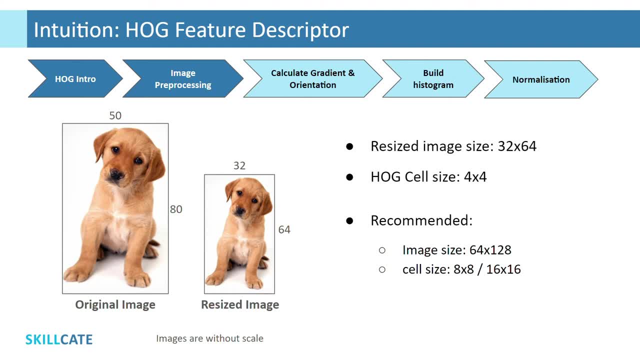 and keep cell size as 8x8 or 16x16.. But in our case the input images themselves are very small. But in our case the input images themselves are very small, So we are using small resize and cell size values. 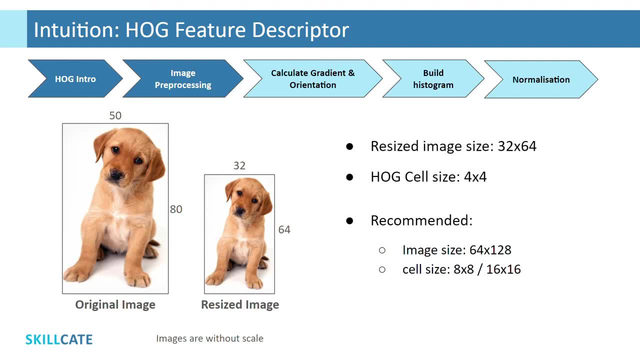 So we are using small resize and cell size values. So we are using small resize and cell size values. Alright, this is the fun part. As we already know, HOG is Histogram of Oriented Gradients. As we already know, HOG is Histogram of Oriented Gradients. 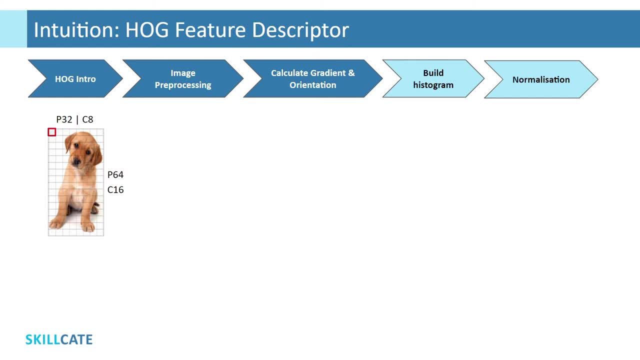 As we already know, HOG is Histogram of Oriented Gradients. In this section we would calculate the gradient and orientation. In this section, we would calculate the gradient and orientation, which we would then plot on a histogram in the next section. 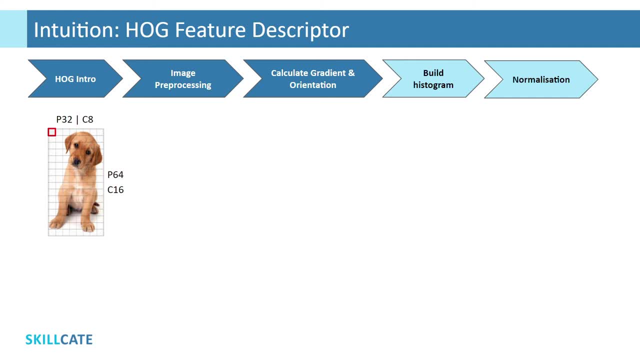 which we would then plot on a histogram in the next section. Here we have divided our image into 4x4 cells. Here we have divided our image into 4x4 cells. As you may see, we have 8 such cells along width. 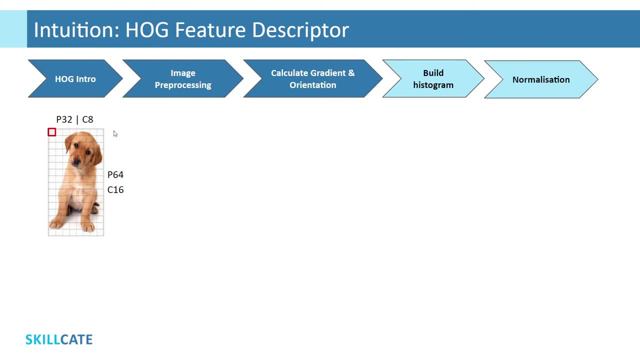 As you may see, we have 8 such cells along width, denoted by this C8, and 16 cells along the height, denoted by C16.. denoted by C16.. For this first cell, let's assume this is how the pixel value matrix is like. 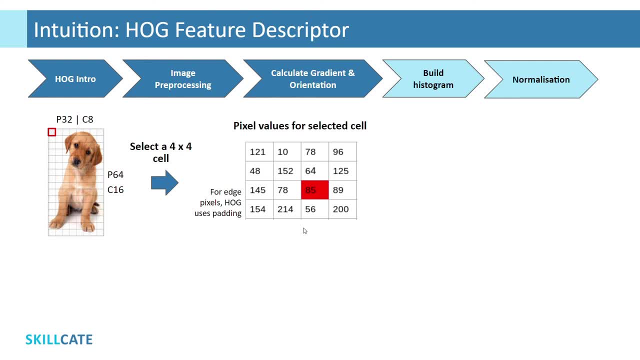 let's assume this is how the pixel value matrix is like. As you may observe, this is 4x4, the way we discussed previously. The first thing we have to calculate is gradient in x and y directions, is gradient in x and y directions. 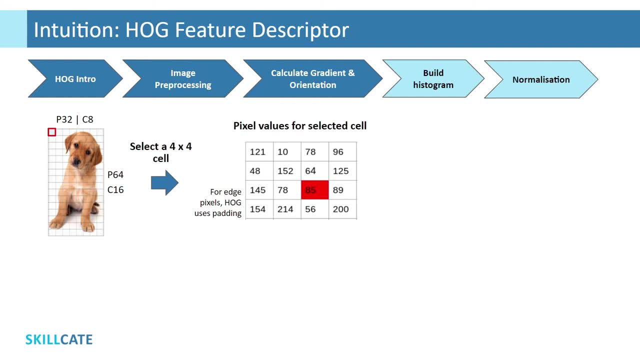 that we call Gx and Gy, that we call Gx and Gy Gradient in x direction, or Gx, is the difference of pixel values, is the difference of pixel values on the right of this highlighted pixel to the pixel value on the left. So this is: 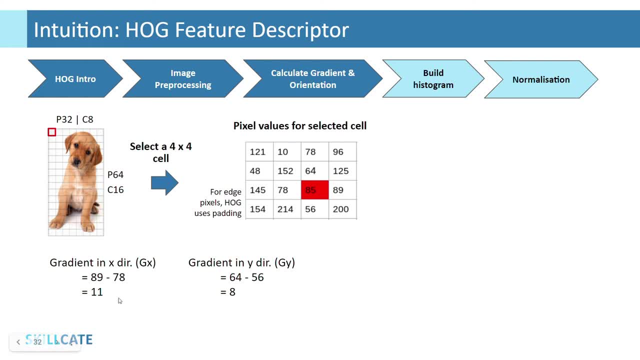 89-78, equal to 11.. Alright, this is our Gx. Alright, this is our Gx. Similarly, gradient in y direction, or Gy, is the difference of pixel values above this highlighted pixel to the pixel value below. So this is: 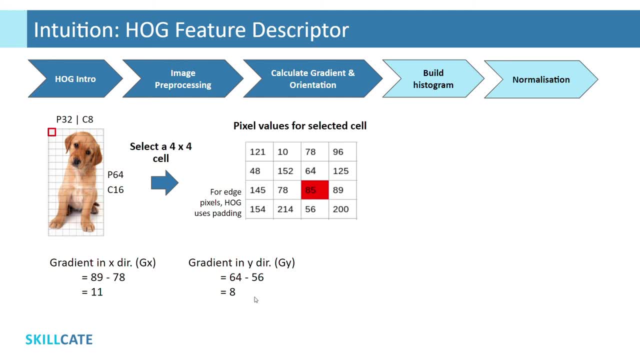 64-56, equal to 8.. This is our Gy. Now, to calculate the total gradient magnitude and orientation from these Gx and Gy gradient components, we would use Pythagoras theorem- Yes, the one we studied in school. So the total gradient magnitude 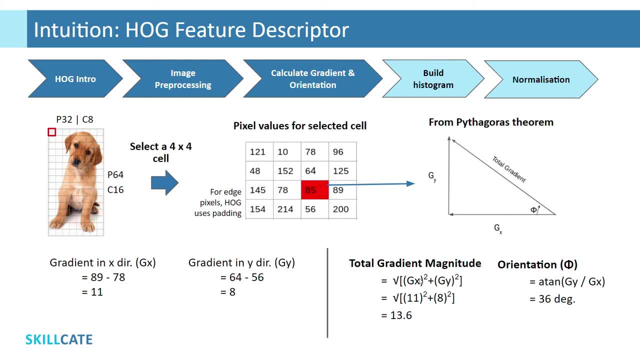 is the root sum of squares of Gx and Gy, which is 14.6.. Similarly, orientation is the inverse tangent of Gy by Gx, which is 36 degrees. Similarly, Hogg algorithm would compute gradients and orientation for all these. 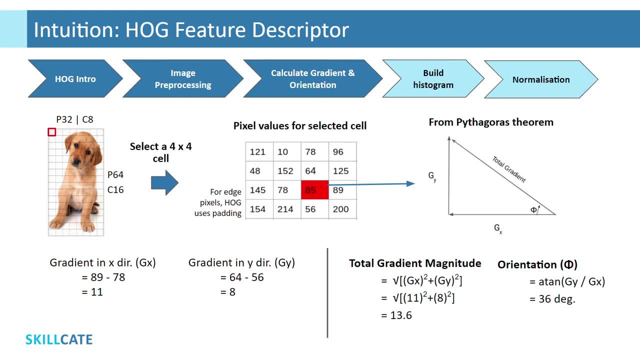 pixels of this selected 4x4 cell. For the image edge pixels, Hogg uses a technique called padding. Please refer to the link in the description part of this video to know more on padding. Next up, let's try to plot these. 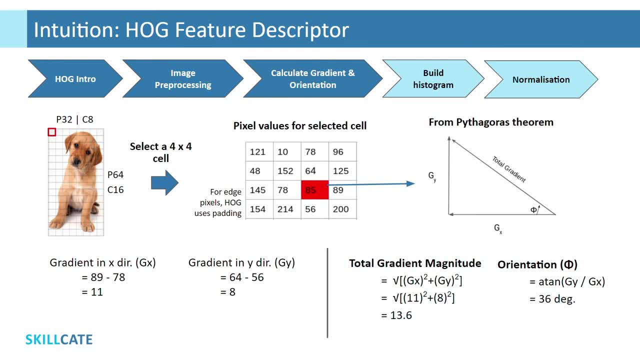 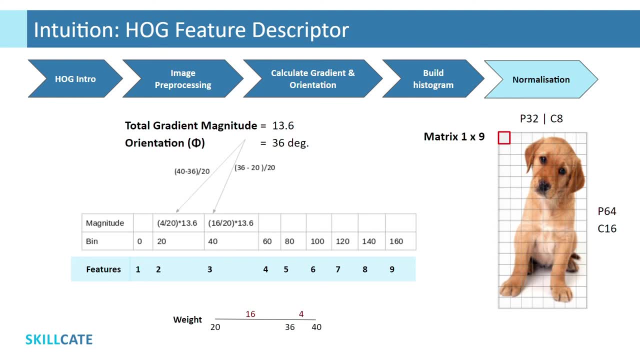 gradient and orientation values on a histogram. Gradient and orientation values for our highlighted pixel are 13.6 and 36 degrees respectively. We already know that this orientation value may vary between 0 to 180 degrees. For the histogram HOG prepares. 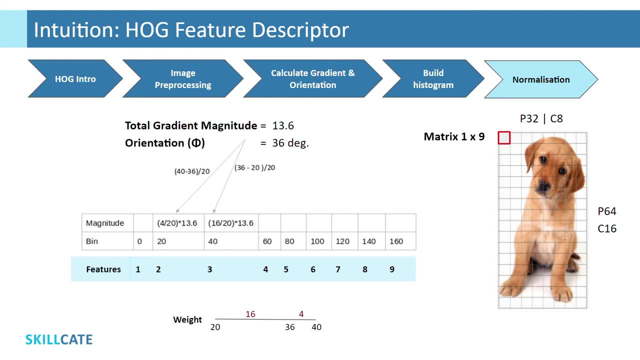 bins of 20 degrees each, So there are 9 bins in total. Next up, Hogg would start inserting gradient magnitude values as per the pixel orientation into these 9 bins, For our highlighted pixel orientation is 36 degrees, which is closer to. 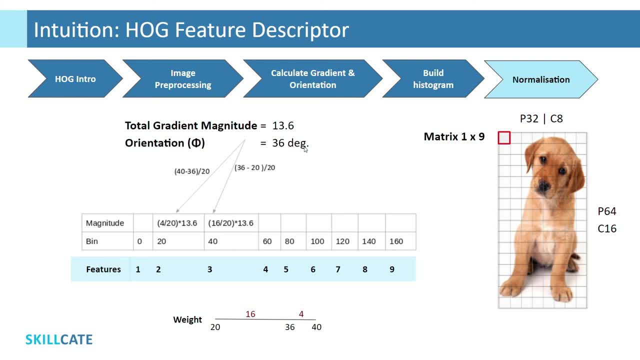 40. So the major contribution of gradient magnitude would go to 40 degree bin and the minority would go to 20 degree bin. We use angle weights to do it. Simply put, 16 by 20 is the weight that is assigned to the 40 degree bin, which is: 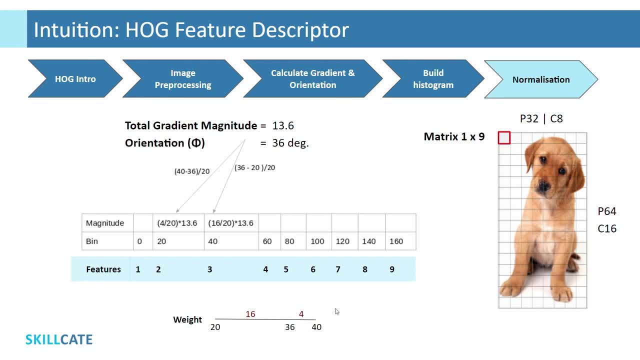 the major chunk of gradient magnitude, and 4 by 20 is the weight assigned to the 20 degree bin, which is minor. Similarly, all other gradient values are added to this histogram based on their pixel orientations for the selected cell Towards the end. 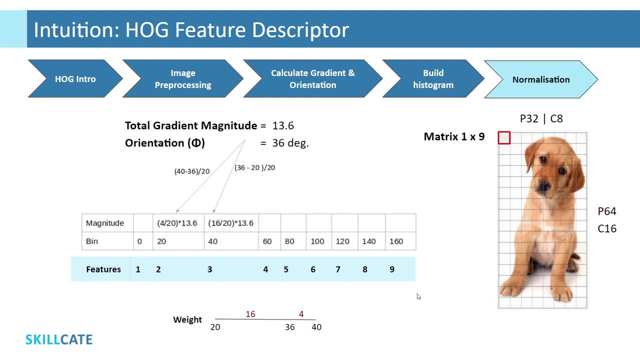 we get a 1 by 9 feature matrix for this cell, Then Hogg would compute such 1 by 9 feature matrices for the remaining cells. Once done, next step is normalization. Localized gradients of image are sensitive to overall lighting.